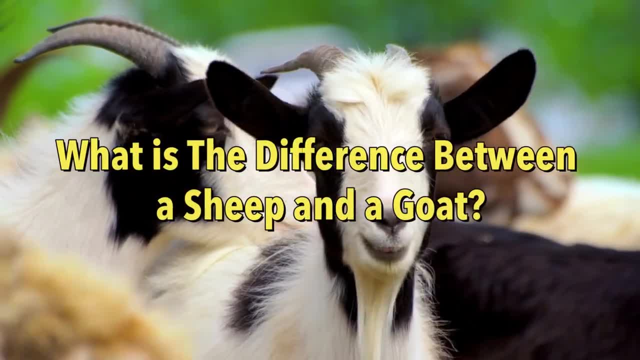 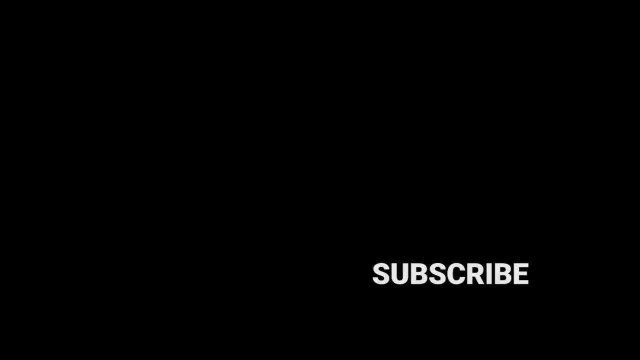 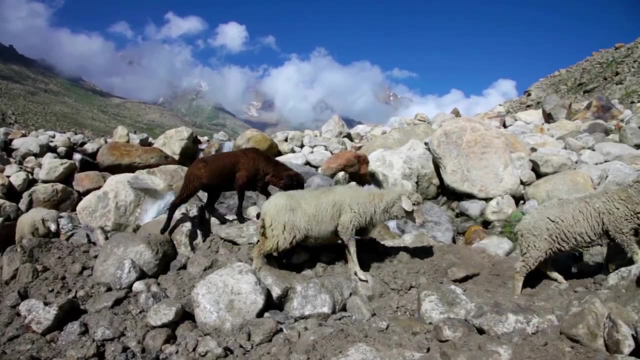 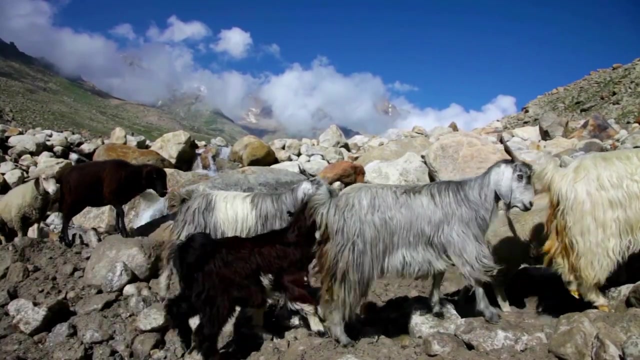 Are you wondering what is the difference between a sheep and a goat? Watch until the end of the video. Well, despite being from the same family group, they're actually very different animals. Sheep and goats have completely different eating habits and different natures. 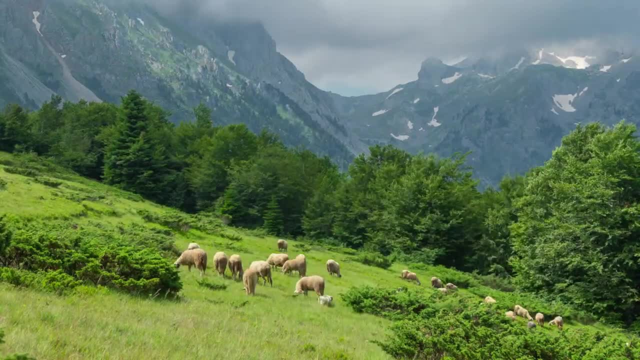 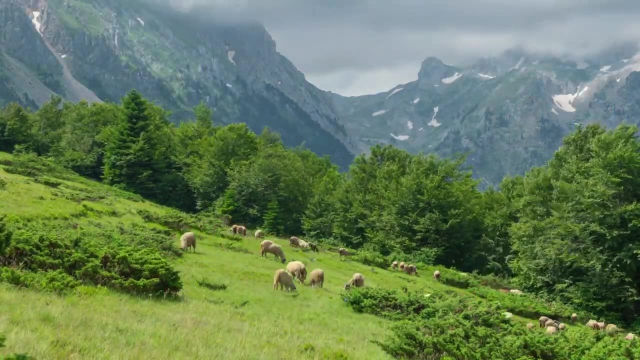 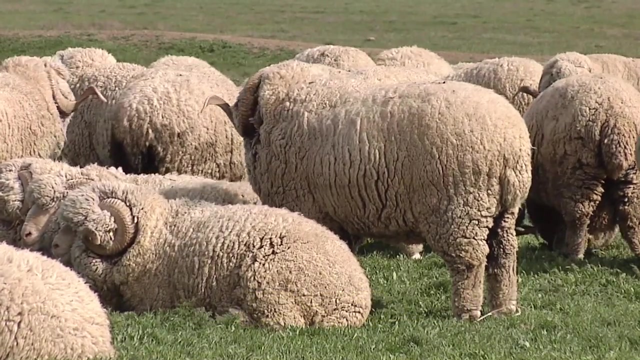 and even different coats. Take a look at the main differences between sheep and goats and find out what makes each animal so unique. Let's get started A fur or wool coat. One of the most distinctive differences between sheep and goats is that they have different 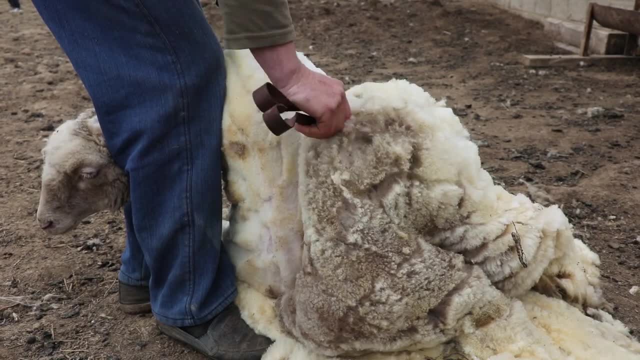 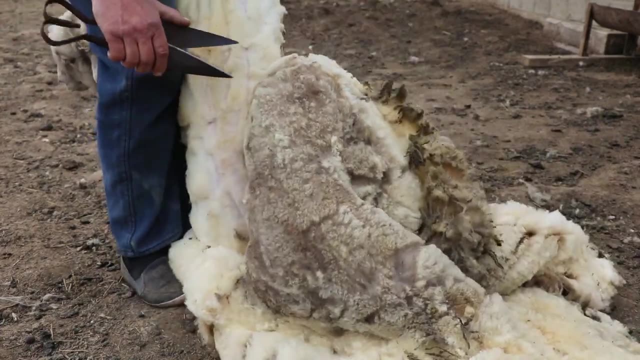 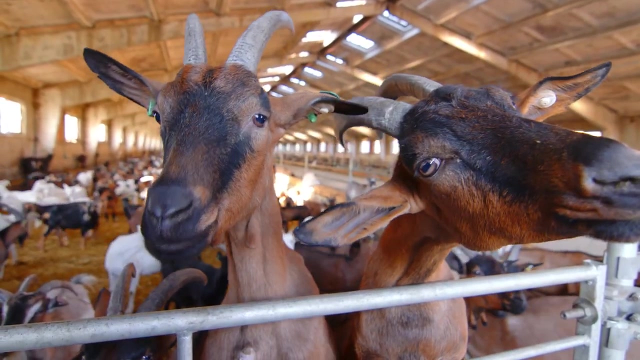 clothing types. Some have wool and some don't. Sheep and goats are known for their wool coat. The only difference between sheep and goats is their coat type. Many types of sheep are woolly and their coats require shearing each year. On the contrary, goats usually have hair coats that do not need regular cutting or shearing. 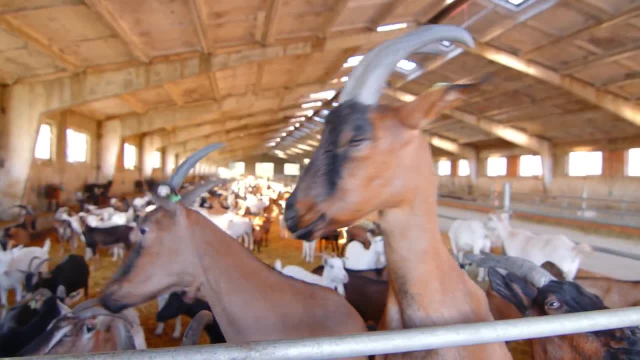 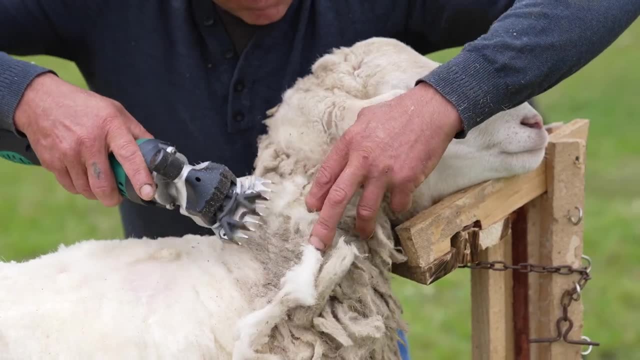 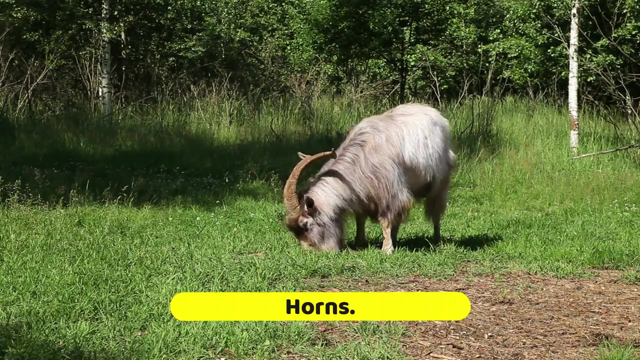 Another significant difference in terms of hair is that some sheep may have manies, while some goats may have beards. After shearing a sheep, especially when they are clean-faced and clean-legged, some sheep breeds can resemble goats Horns. More often than not, goats have horns. that 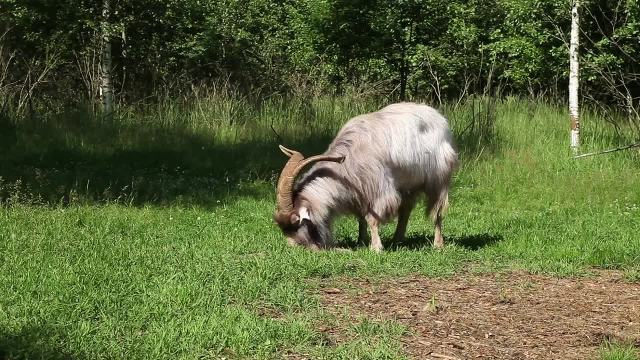 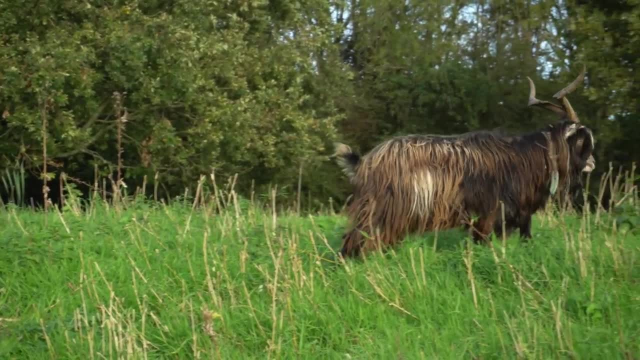 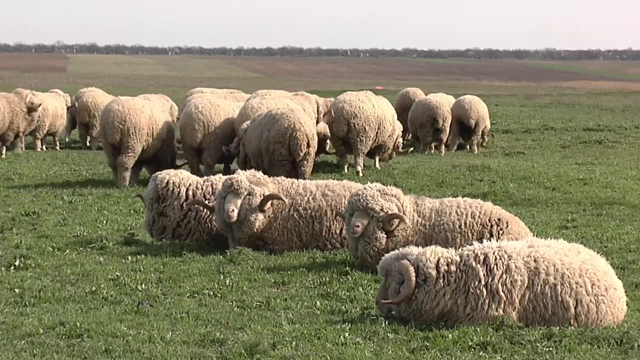 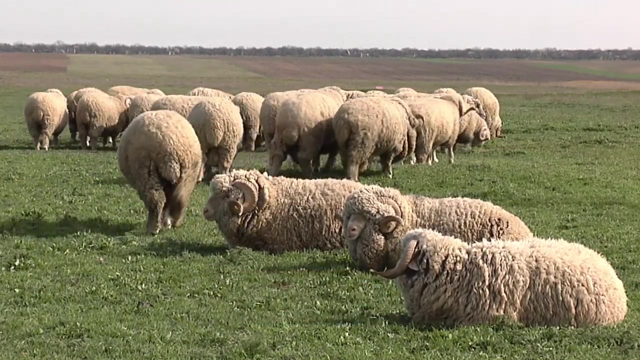 are usually narrower and straighter than sheep horns. They also usually point more upwards and back and don't curl round. Most sheep- although not all- are naturally pulled, which means they don't have horns. However, of those that do, their horns are usually thick and curl round impressively. 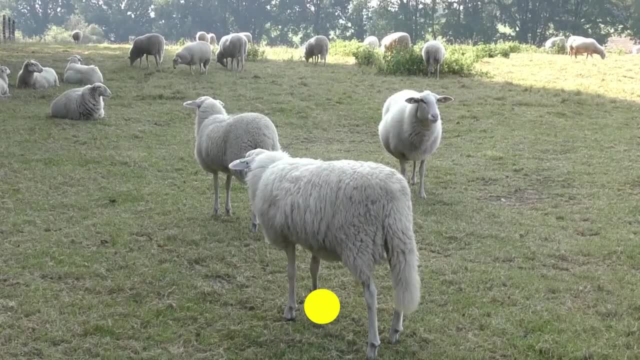 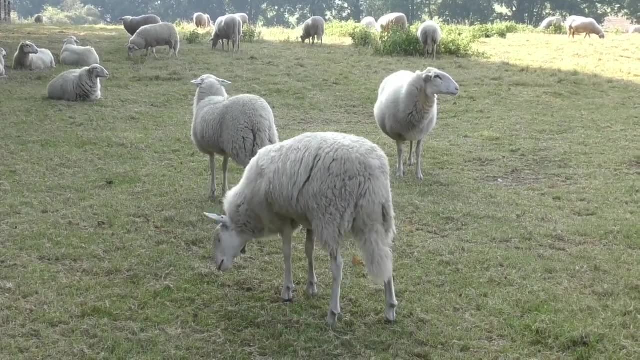 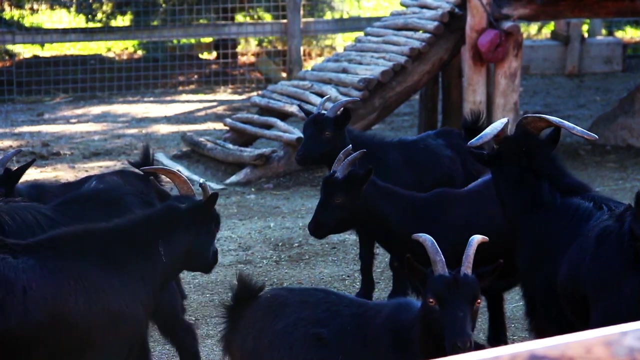 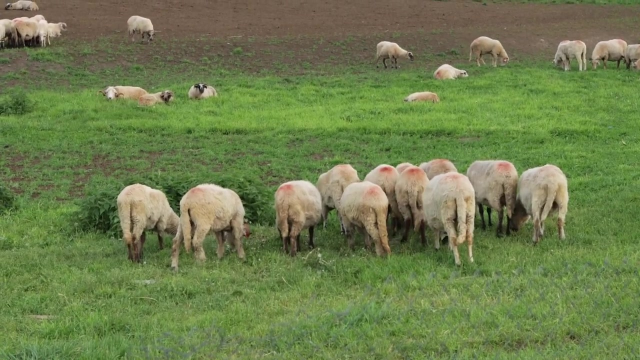 at the side of their heads. Tail Pointing The tail is often considered the fastest way to see the difference in the goat version. Goats have short tails that are usually pointing upwards unless they are scared or ill. On the contrary, sheep have tails that point downwards. Most sheep are born with long tails that are docked at birth for sanitary reasons and to help prevent fly strike. Long tails often get covered in feces, which attracts flies. Fly strike is then caused when blowflies lay their eggs on the back of the sheep. 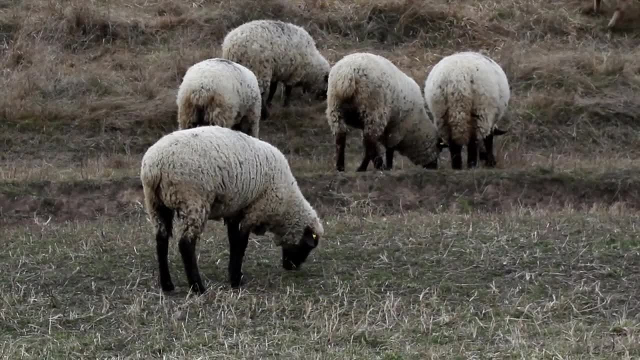 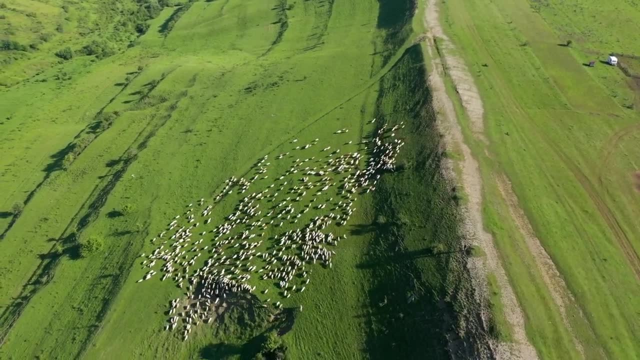 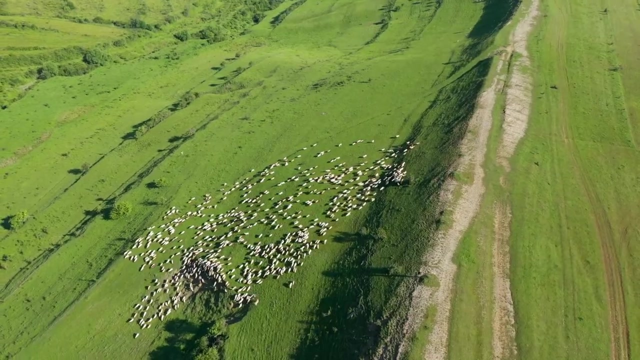 Personality, Temperament. Sheep are best known for their relatively aloof and distant behavior and their strong flocking instinct. Sheep are more mellow than goats, since they prefer to eat what is on the ground and only graze to eat what they can see there. 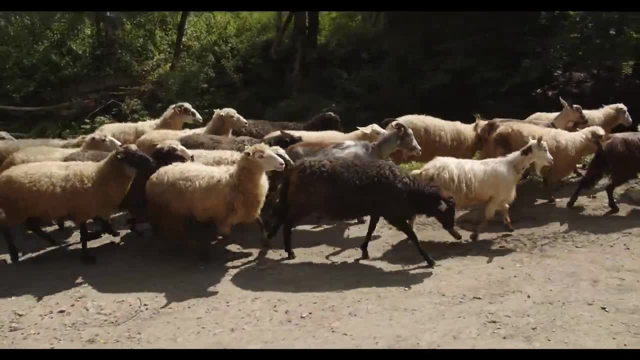 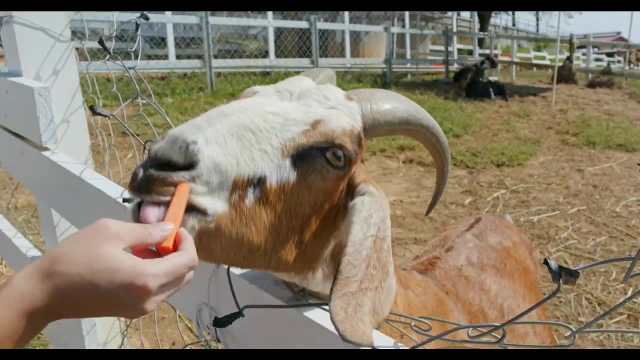 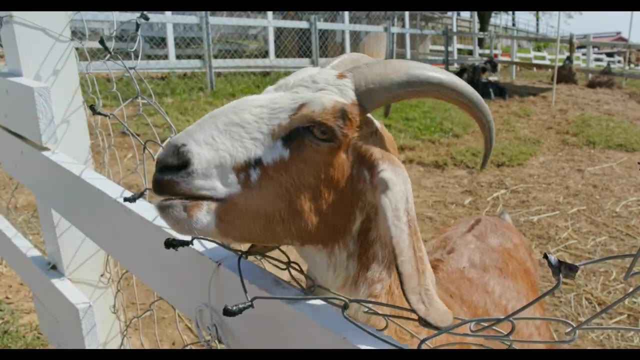 When they are under threat or weathering a storm, they will naturally flock together into a group and can quickly become distressed when separated from others. Goats are usually considered more independent, curious and troublesome. since they love to explore, They are very curious about their surroundings and will interact with their environment to 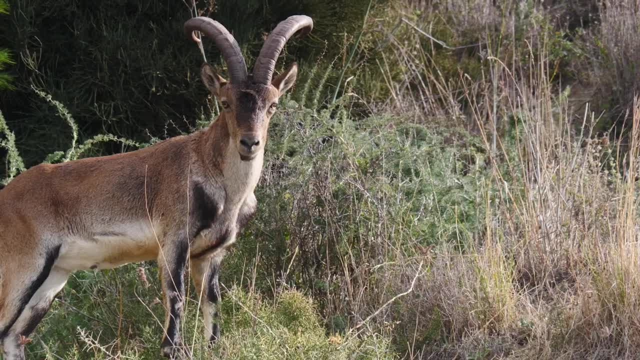 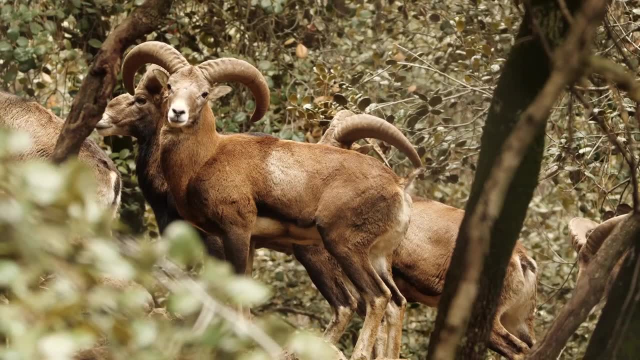 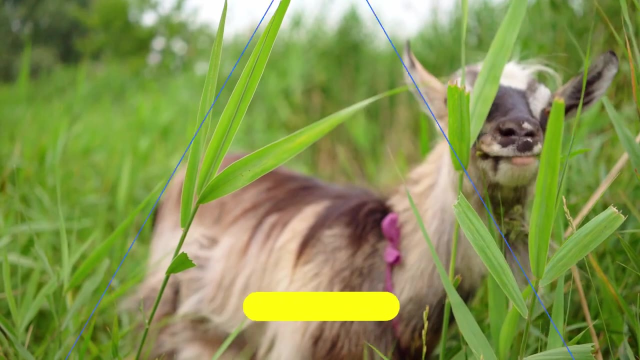 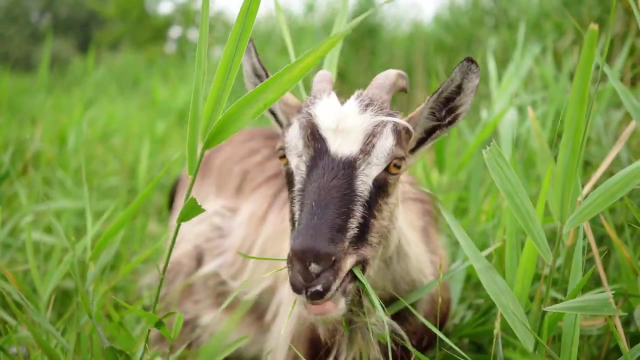 a high degree. Goats are extremely agile and are well known for their ability to jump or climb things, but it takes good fencing to keep them in Eating Grass or Trees. Goats prefer to eat leaves, twigs and shrubs and often stand up on their hind legs to reach the tops of plants. 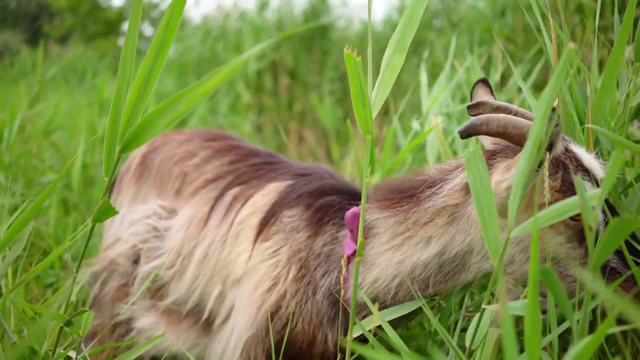 However, coupled with their curious and inquisitive nature, their liking for anything they can get in their mouths often gives them a bad name. They are also known for their strong sense of smell and taste. They are also known for their strong sense of smell and taste. They are ofteneted by their strong sense of smell. They tend to avoid burning dishes, but smell the food first and then eat it after a while, While, on the other hand, sheep are grazers and prefer to eat from near the ground as they graze while they wander around. 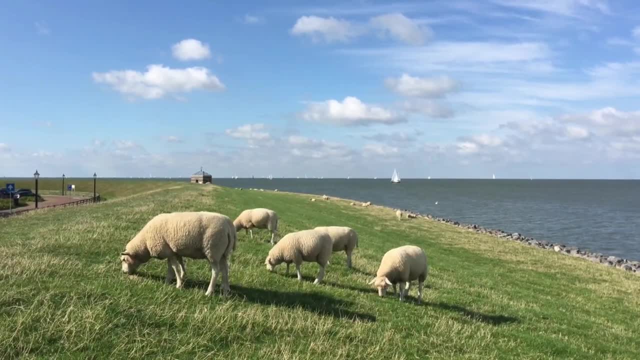 In general, cows are like the ones they eat. They tend to eat grass, need to feed on it and their own food. They get their meat and meat to eat in the morning, and even their own food, While, on the other hand, sheep are grazers and prefer to eat from near the ground as 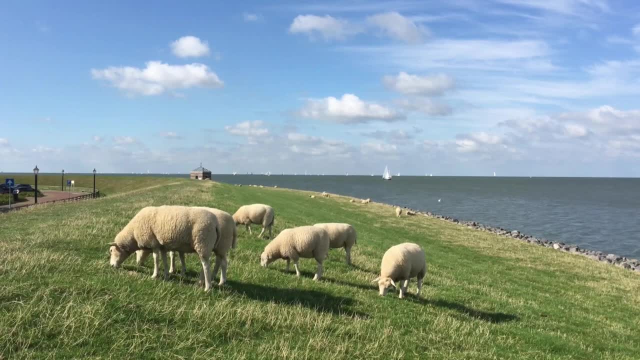 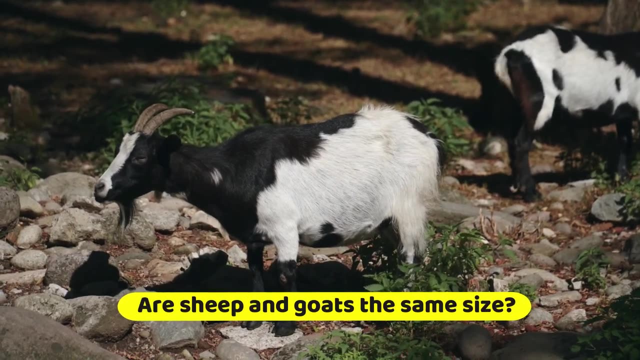 they graze while they wander around. Sheep usually eat short grasses and clover and largely ignore trees and shrubs. Not to mention, goats tend to eat short grasses and clover and largely ignore trees and shrubs. Are Goats and Sheep the Same Size? 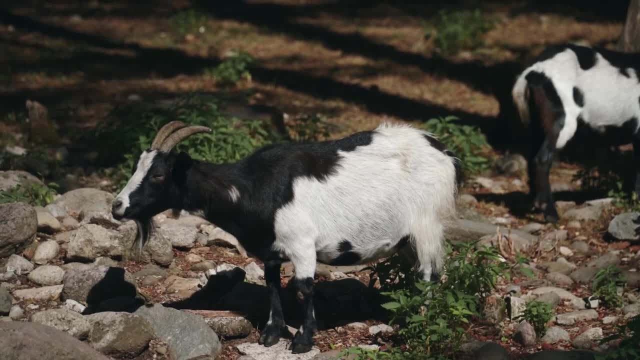 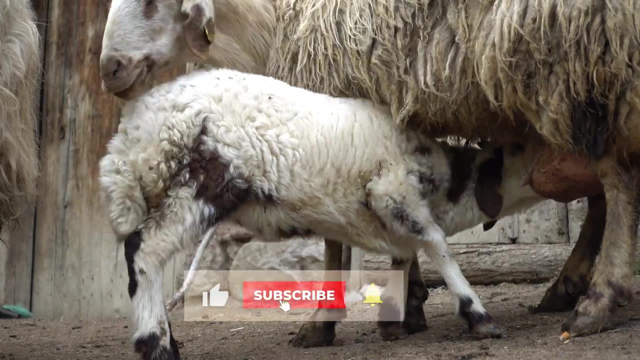 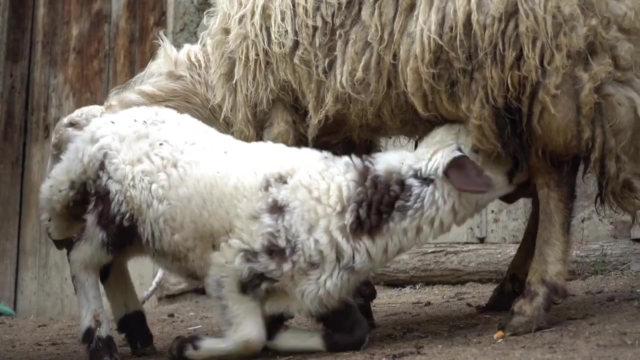 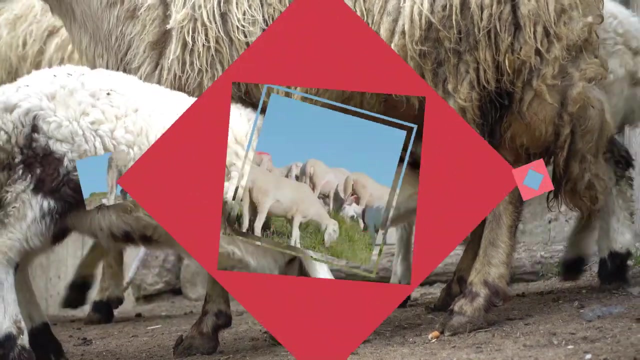 There can be a vast variety of sizes in both sheep and goats, but generally, to look at, goats appear to be slimmer than sheep, As well as being because of their woolly coats. sheep process their food differently to goats and so generally put more weight on across their loins and backs than goats do.